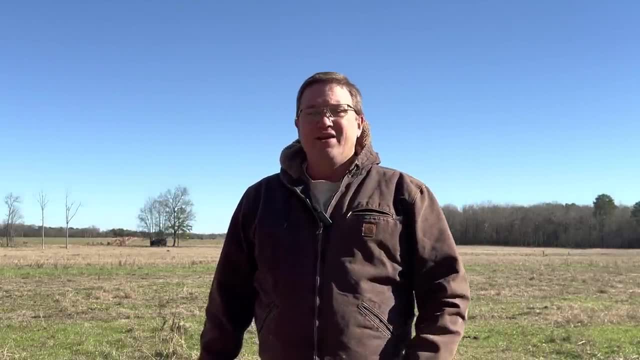 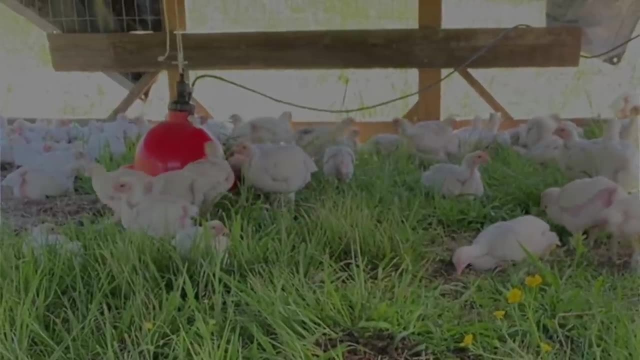 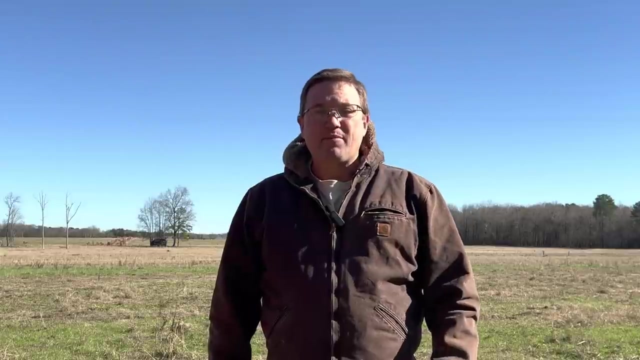 of your soils is by using livestock. Now we've run meat chickens and egg layers on our farm over the last several years. We stopped doing this two years ago, but it's amazing how much fertility the chickens bring to the farm. The problem that we ran into is doing this on a smaller scale. You 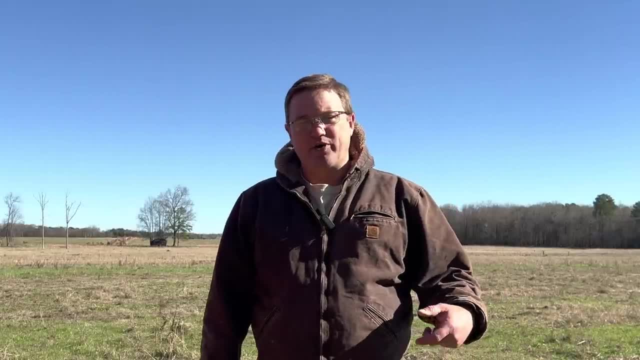 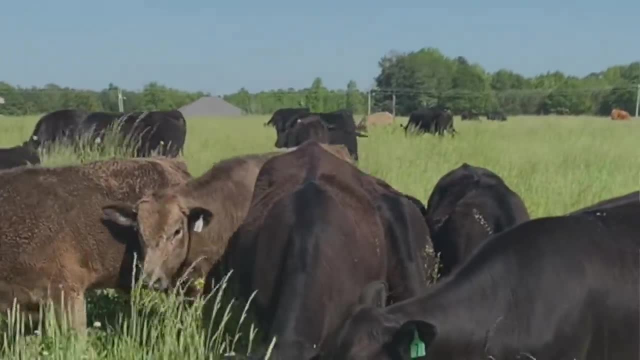 spend a lot of time, energy and effort doing it, and so we've focused primarily now on pigs and cattle. If you manage ruminants and small paddocks, it's called management, intensive grazing or rotational grazing. They'll trample a lot of the 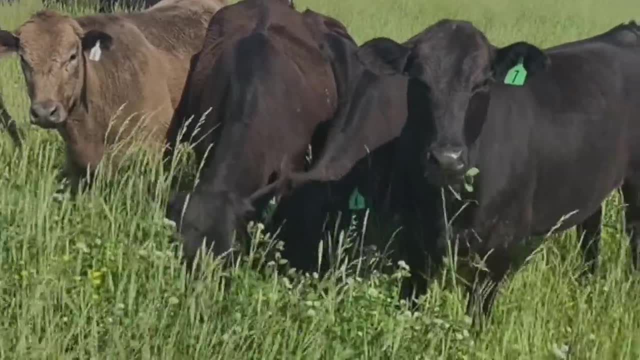 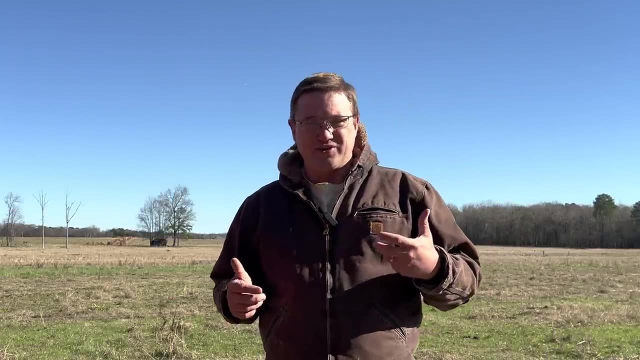 weeds and stuff that they don't want to eat, and then they'll graze the good products and then you move them the next day. It creates a lot of great soil health. The second strategy that I'll mention is using cover crops in your soils. You can plant them with a no-till drill and they won't mess up. 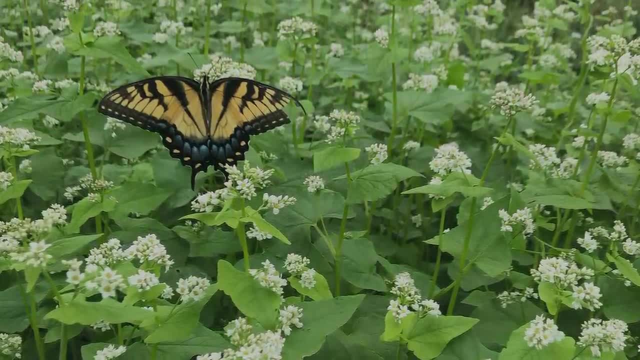 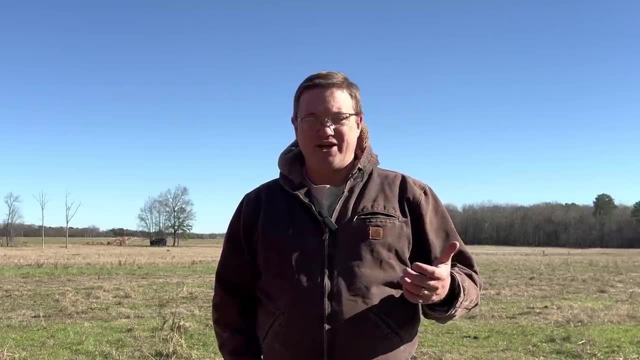 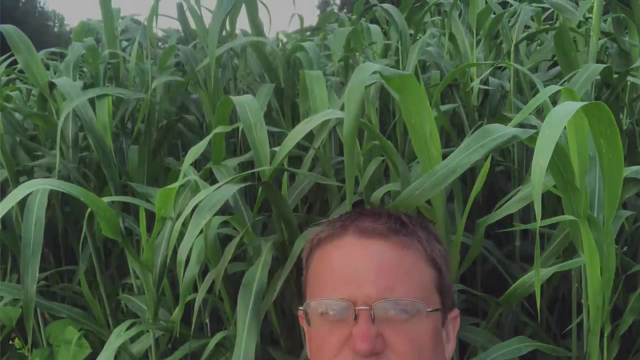 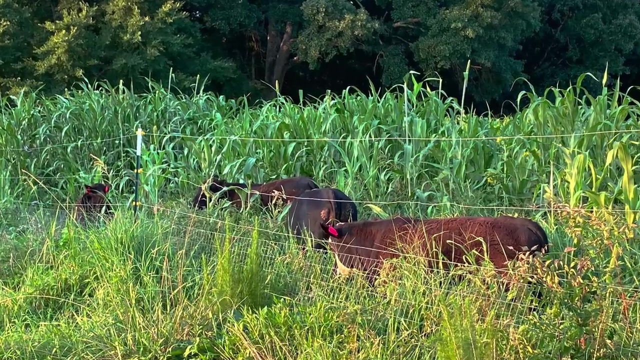 your sod and it is amazing how much organic matter just one growing season of a sorghum grass-based cover crop mix can put into the soil. They can grow anywhere from six to 12, maybe even 14 tons of dry matter per acre. That is huge. However, the downside of that is getting it planted. 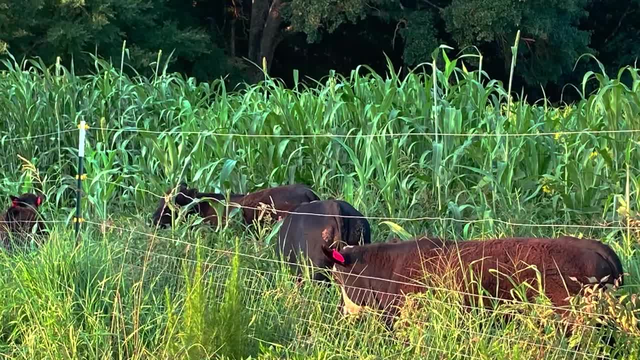 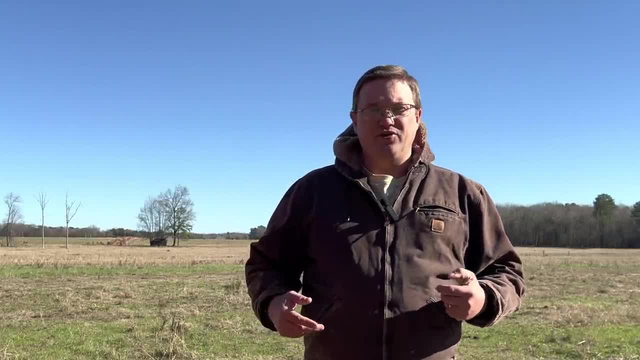 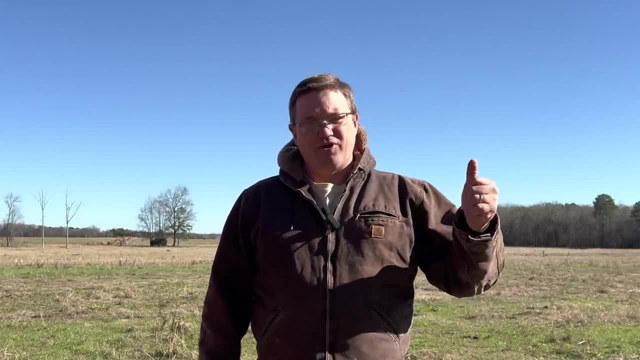 on a hundred acres is really really problematic. We'll come back to the problems with some of these strategies in a few minutes. The third primary strategy that you can use is apply carbon directly to your soils. There are a lot of different carbon bases that you can use from. 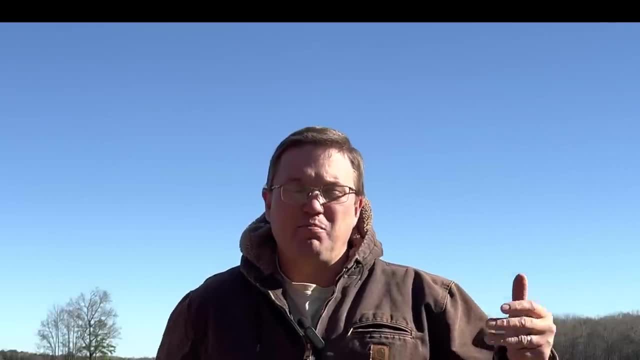 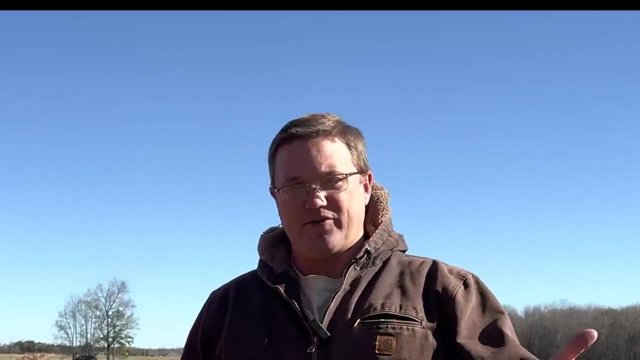 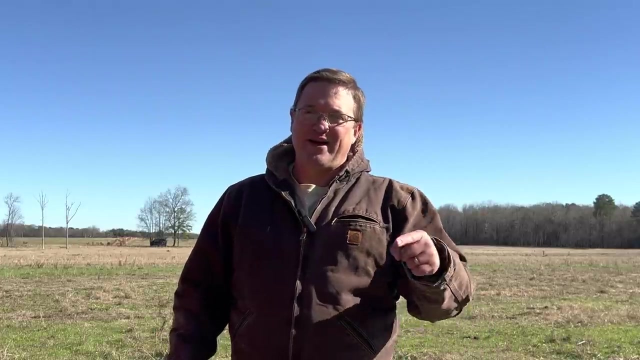 hay to mulch hay, to leaves to compost biochar. There are just a whole lot of different types of carbonaceous materials that you can add to your soils to increase their fertility. They have their downsides as well. So come along and join me as we talk about how we've done it on the farm and how 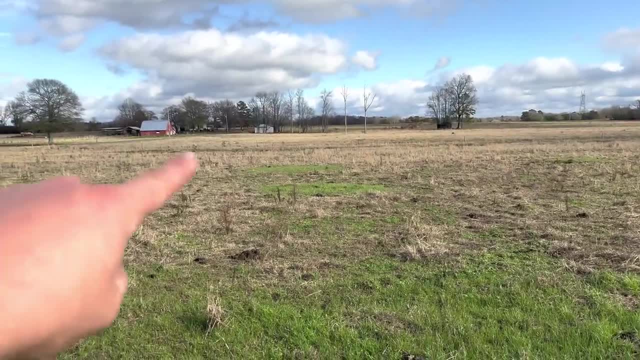 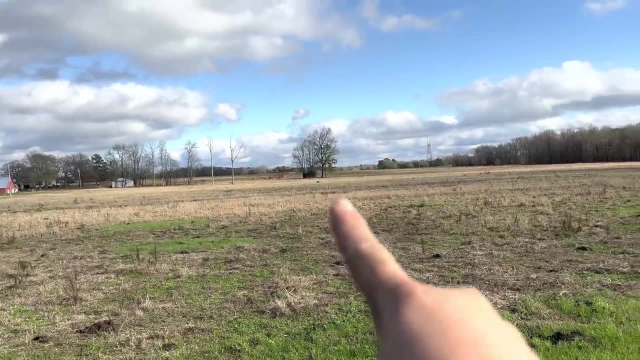 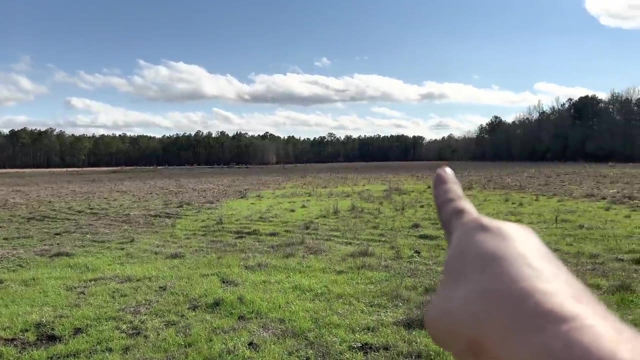 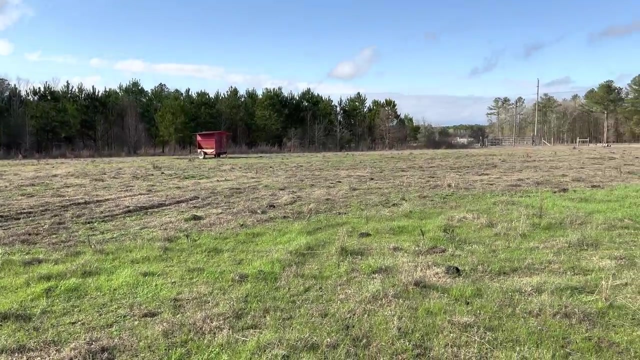 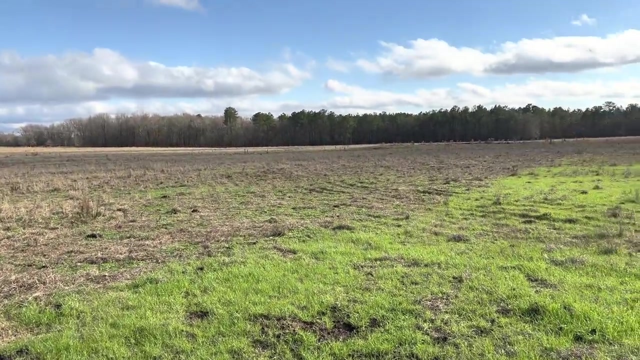 you can do it as well. So my dad cleared this field. It was originally in some kind of scrubby mix field. it was going up to a behind the grain standard. This is where our versuchen that width line, And I just showed this. 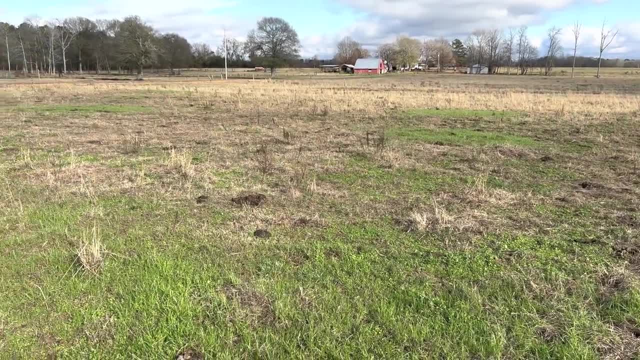 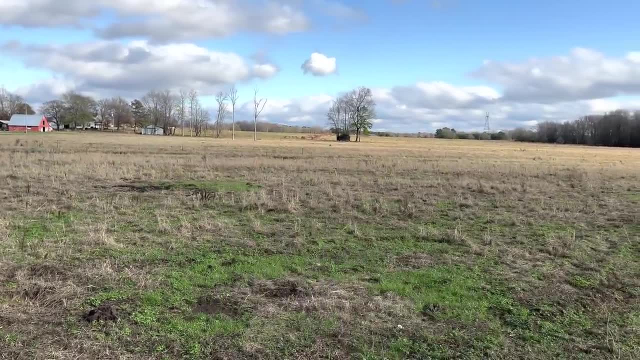 But leave the green fur thawing out Now. so the reason why is for fresh water, housing costs dwindling, have a whole lot of real good summer grazing. On the other side of that little short line of trees closest to us, where the barn and that shed are, is what we call the redfield. 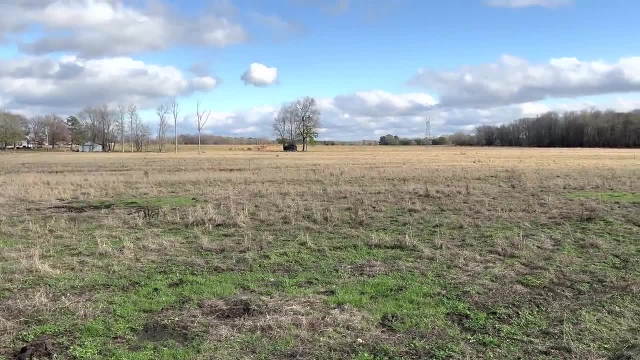 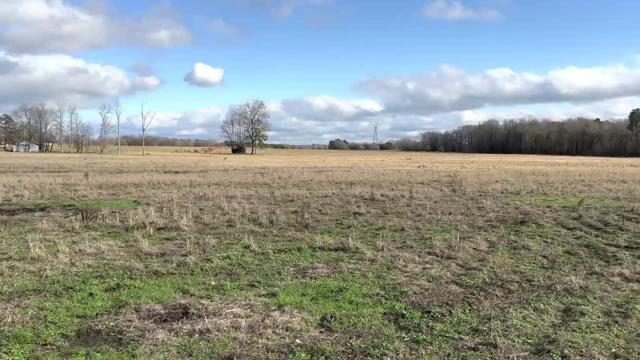 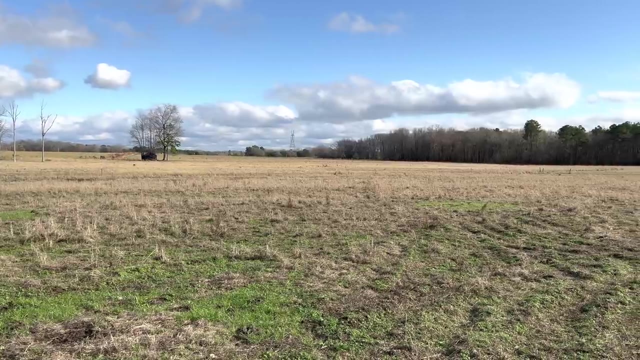 and it's about 50 acres or 40 acres, I forget now which, but in the redfield it is. it has a good stand of fescue and a good stand of white clover, and we've scattered some dock and chicory plantain over the years in there as well and it performs really really well. 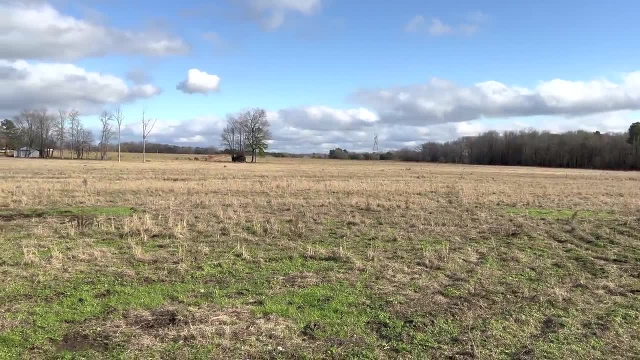 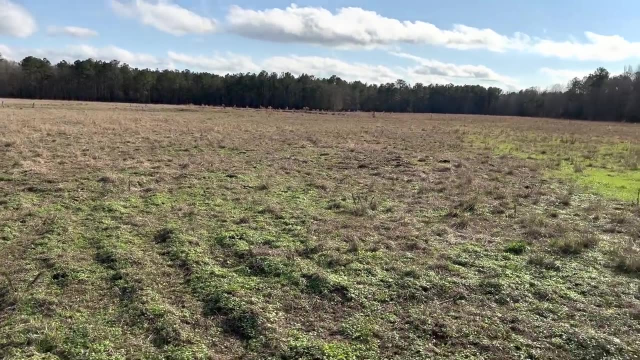 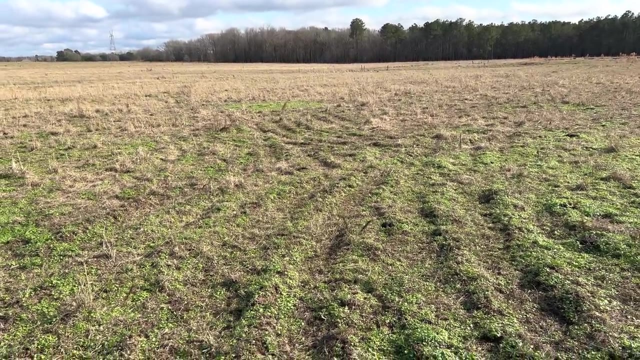 especially in March, April and May. those times of the year it just performs better than any of other pastures. And this so we this. we just use a summer grazing. it's wet and so in the summer it tends to dry out some when we have less rain, and so we move the cows in here graze it. 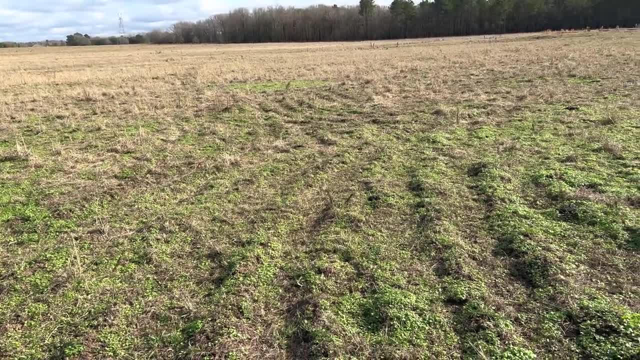 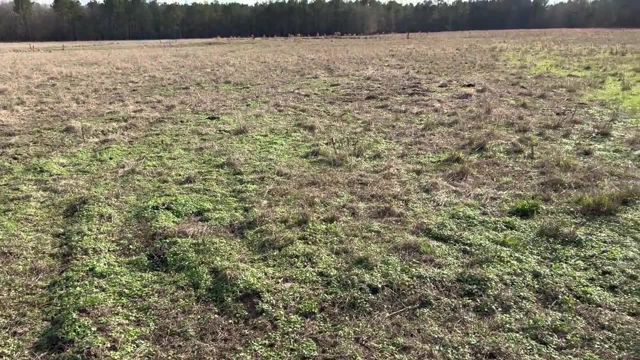 really well and we've got a lot of redfields hard really fast. Move the cows off of it, let them re-graze it. We get a lot of what's known as weedy grass. There's no real good Bermuda, no other real good. 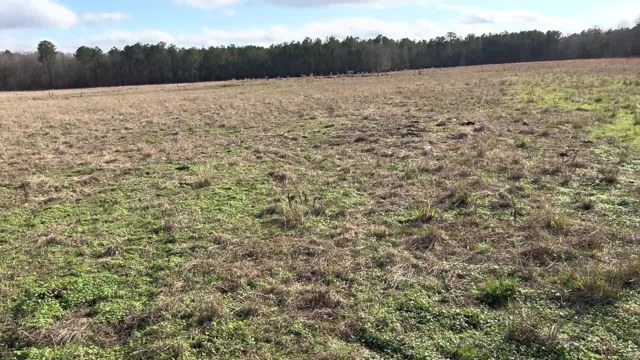 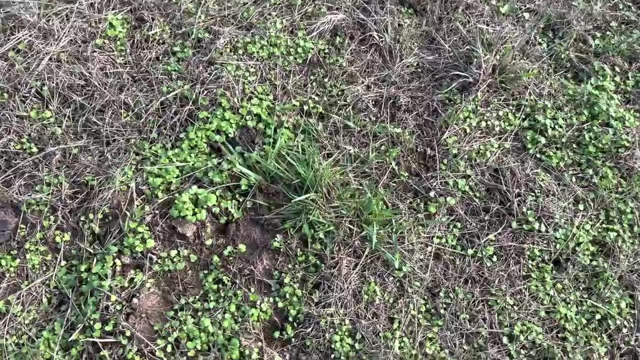 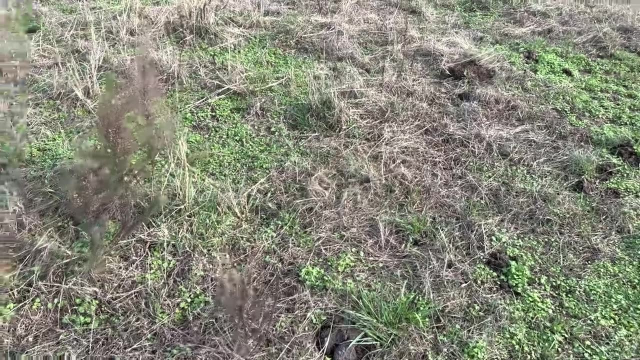 grasses. The cows eat it and perform pretty well, and even if the soil is acidic, that's fine. There's a little bit of fescue, as you can see in that little clump of grass right there, And you can see little spots of fescue here and there. So there is a little. 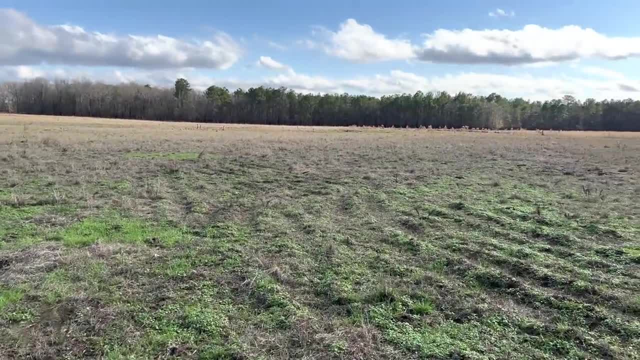 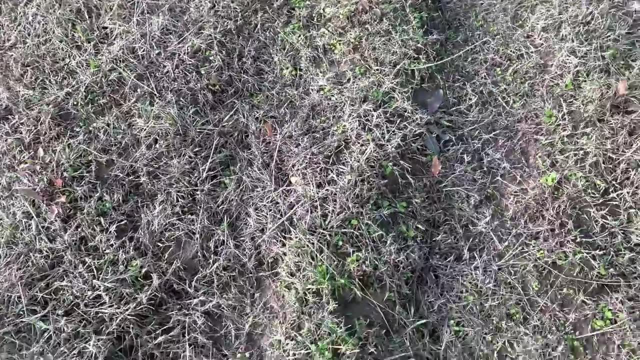 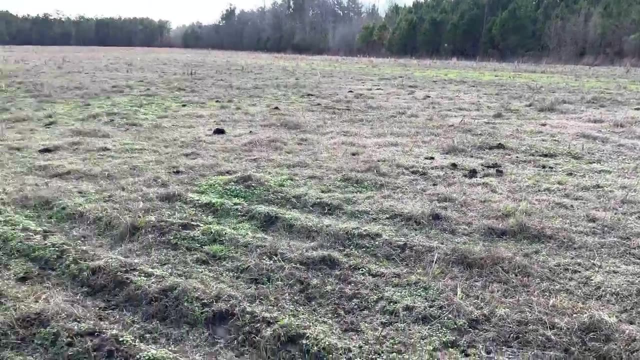 bit of descent- cool season forage, but it's very slim pickings. We fed hay in this area last year. In fact, you can still see tractor roots right here that are three or four inches deep. They're not real bad, but it's a very uneven. 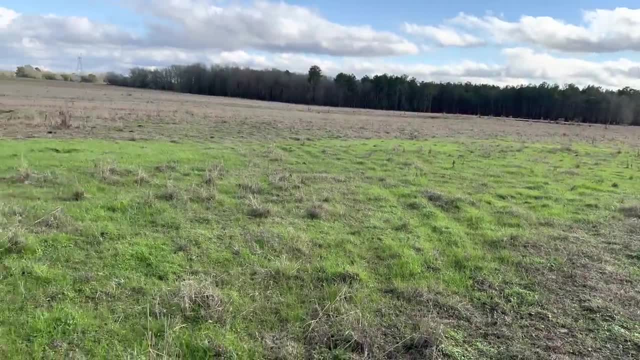 ground Where we fed hay last year, I scattered some ryegrass seed, along with some peah. *** Louder Jingle ***. That's it for this video. Get a check of all of the 86 runs that I've done on this channelうわaa. 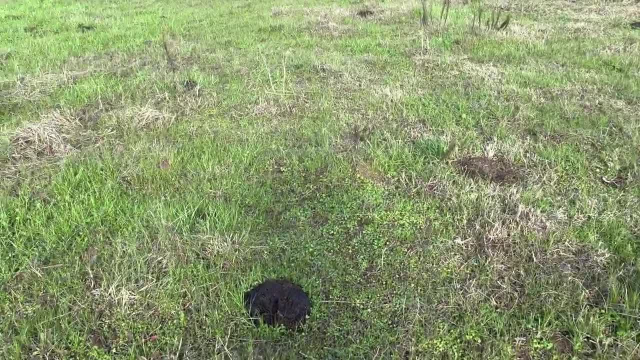 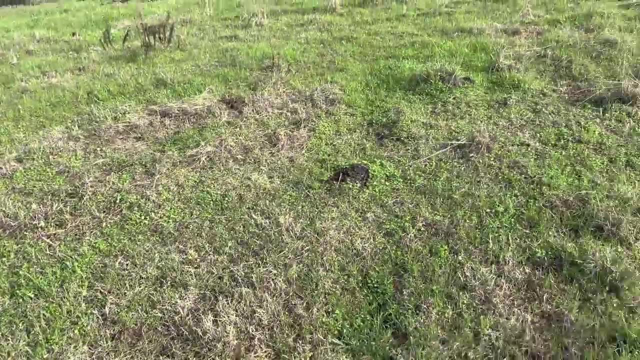 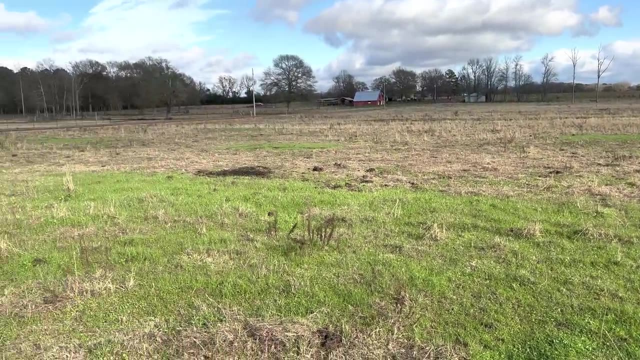 some clover seed and it has taken off and performed relatively well. Cows were over here about three weeks ago, so it's had some moderate success and you can see additional areas, little spots of green where we had fed hay as well, but here the primary strategy is just keep. 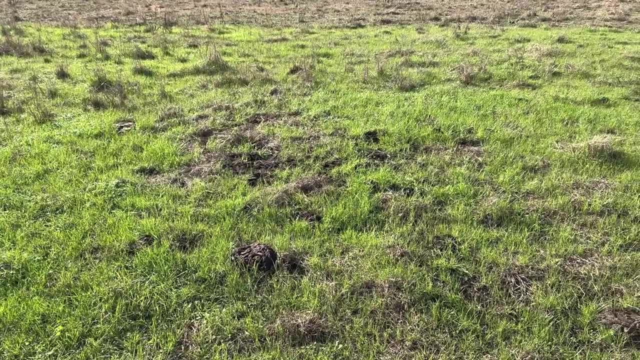 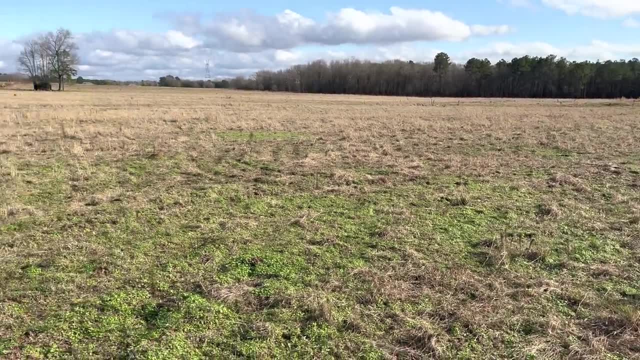 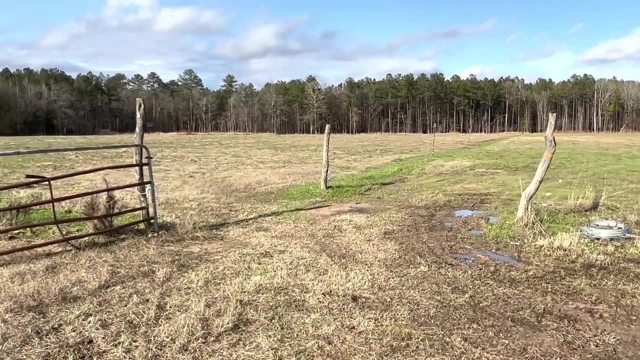 keeping the cows out here. I'm also working to improve a 10 acre field- poor soil, kind of wet, just like this across the road, so let's jump over there and see what it looks like. So these three wooden posts here are the gate systems for the entrance into this 10 acre field here north of. 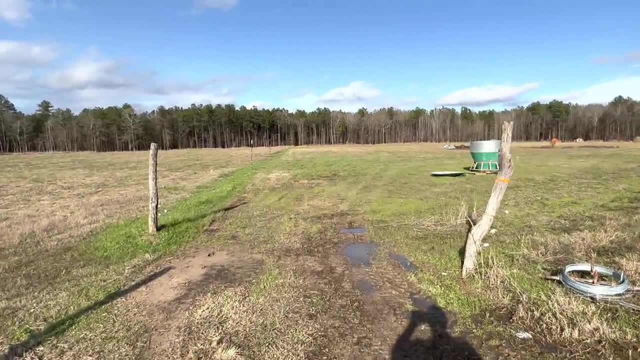 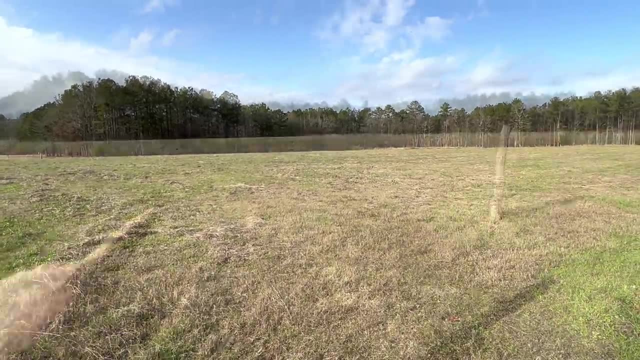 Dowdle Road. Over here to the right I've had pigs in this paddock before. it's about five acres, and in this paddock over here I have nine cows. I've had pigs in this paddock before. it's about five acres as well. The paddock over here to the left is what I'll call paddock A. It is on the edge of. 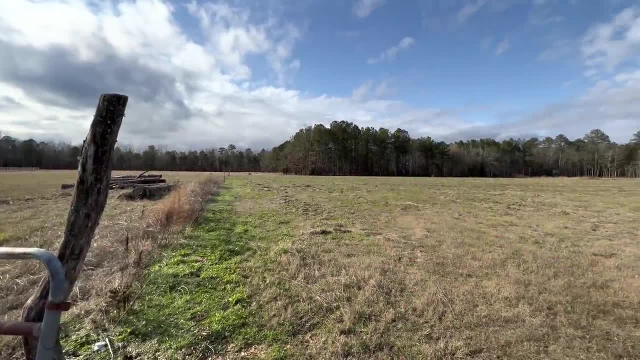 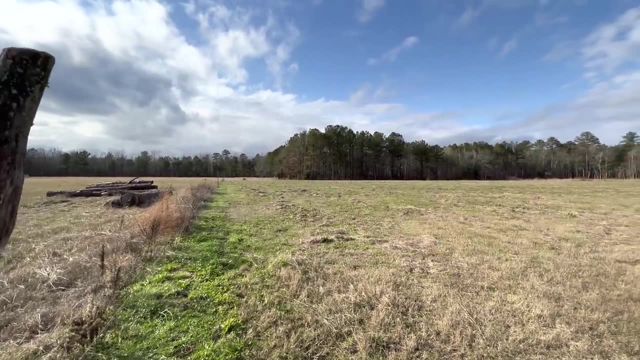 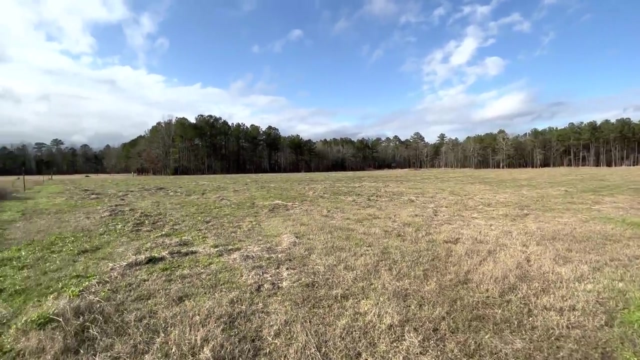 the property. This southern fence and that western fence do not have good pig fences on there yet, so I've got to string up some wire to keep the pigs from getting out over there. However, the northern and the eastern side of paddock A are fine for pig fences. 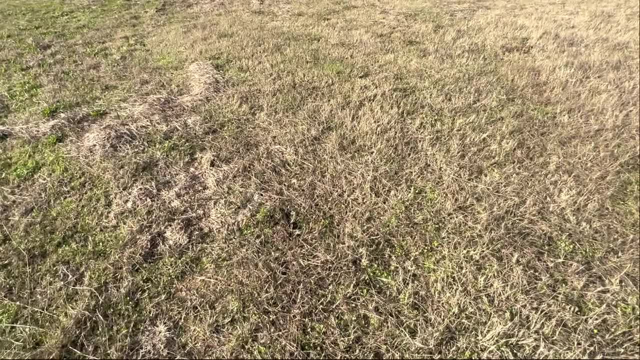 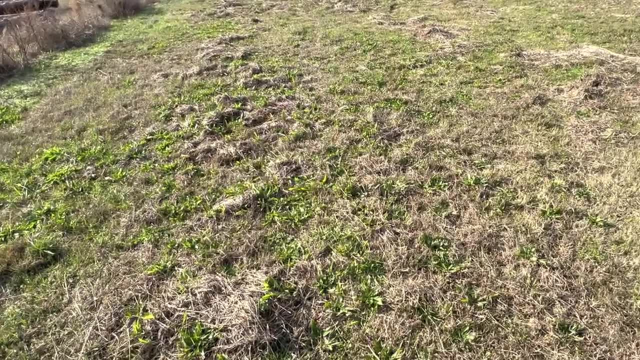 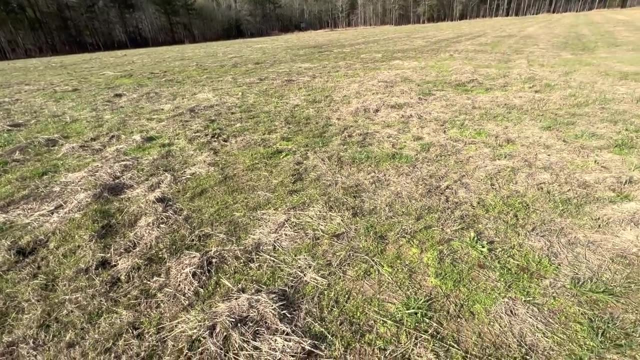 Mostly what's growing in here now. you see some Bermuda at all right here at the entrance. We see a good bit of plantain right here. when you first come in I did broadcast some rye grass and clover over here so you can see the little bits of thin grass growing. that's the rye grass. 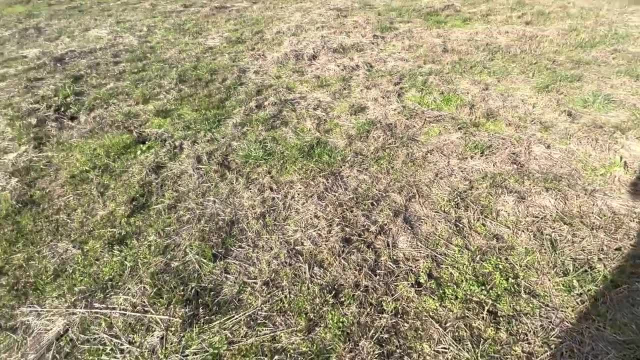 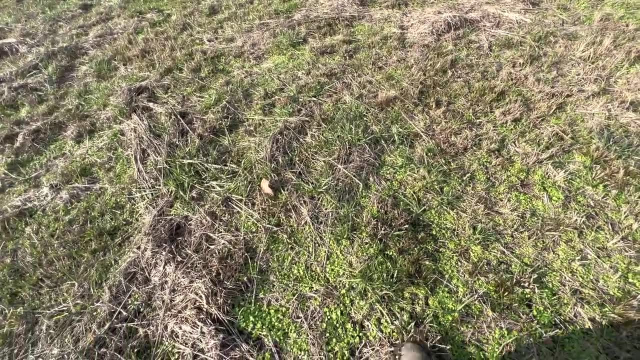 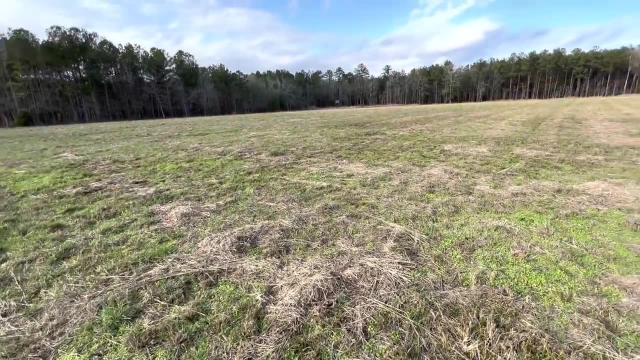 See a little bit of clover- that may be what has already been there- and you can tell that most of the grass is still growing. And then you can see a lot of stem grass. here There's some fescue, but there's also some broom sedge and a lot of just weedy, coarse, tough grasses. Vasey's grass is in. 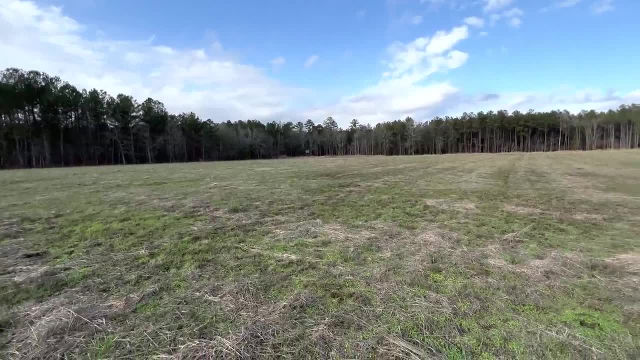 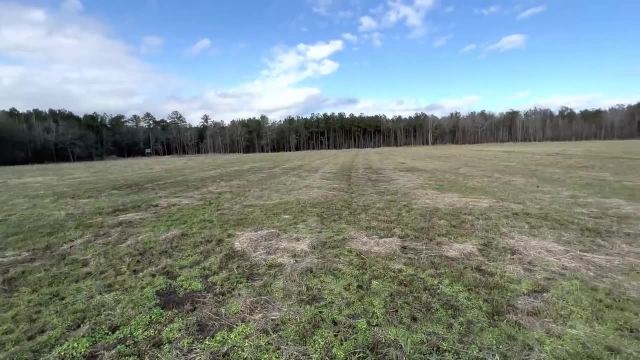 here and it's similar to dallas grass. It's just not the most productive or the nutritious for livestock. Pigs will eat it, but it doesn't really do anything for them. but in this field we've only had cattle grazing. I do want to put pigs in here. I'm not sure at what point I will do that. 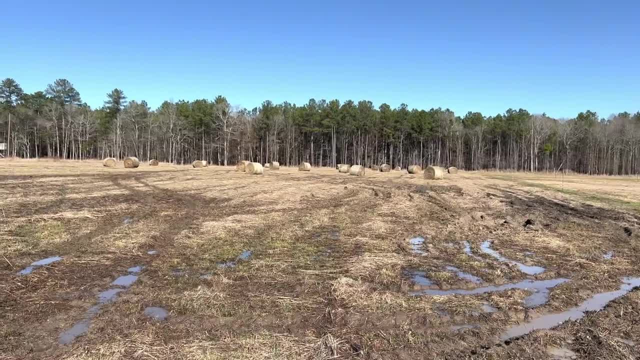 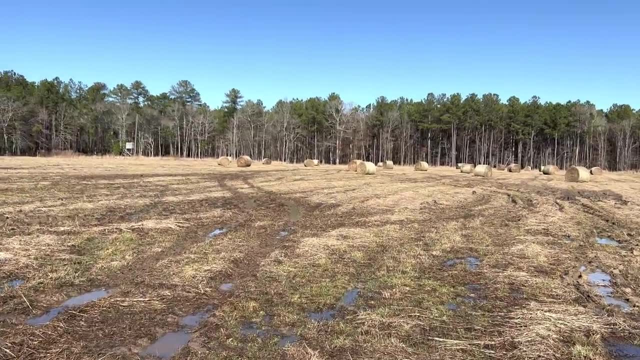 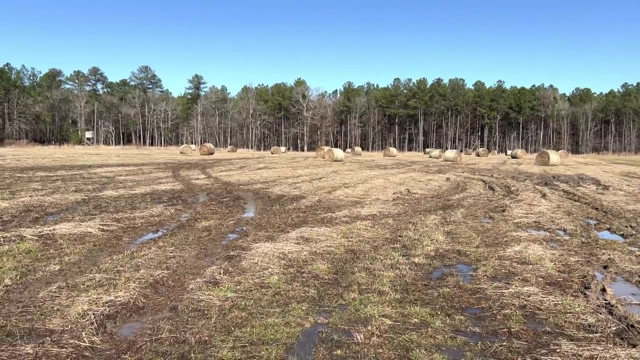 that, but it will be easy to do so. it's been a week and a half since i recorded the description of this field. this is paddock a. each year we feed 50 to 100 bales of hay. we're working to graze a little more efficiently, but this year it looks like we'll be feeding 50 to 60 bales of hay. 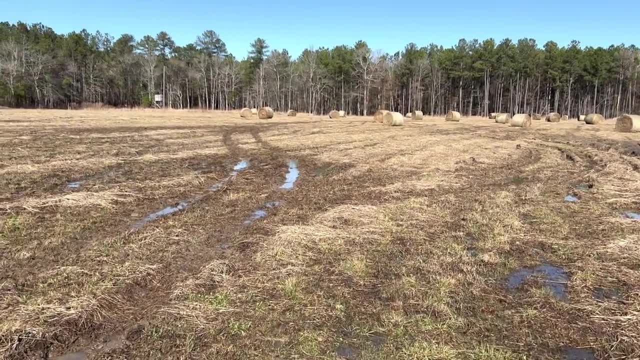 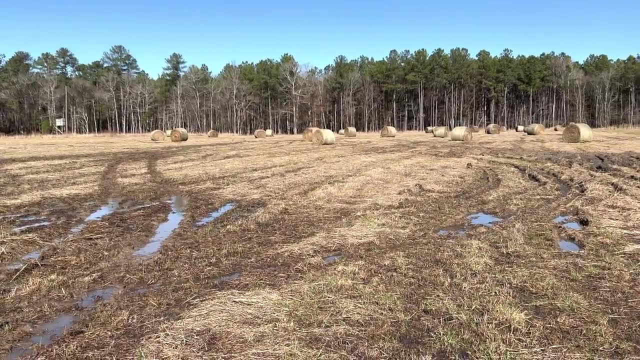 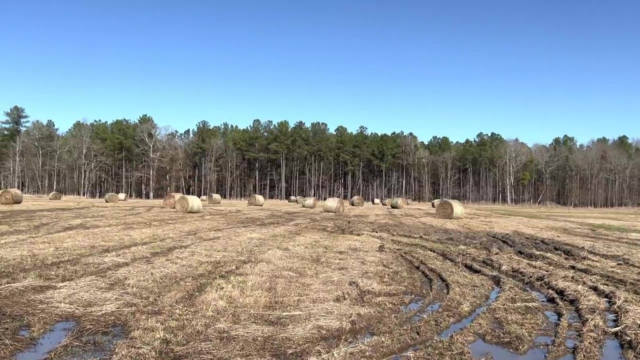 we've had about 30 of those bales of hay delivered so far. the guy delivering the hay got stuck and that was very interesting and i've just placed these bales of hay at different areas around the field. we've only got about half the hay delivered so far, and what we're going to do 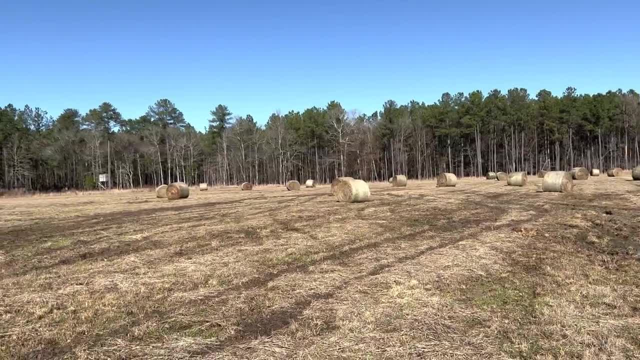 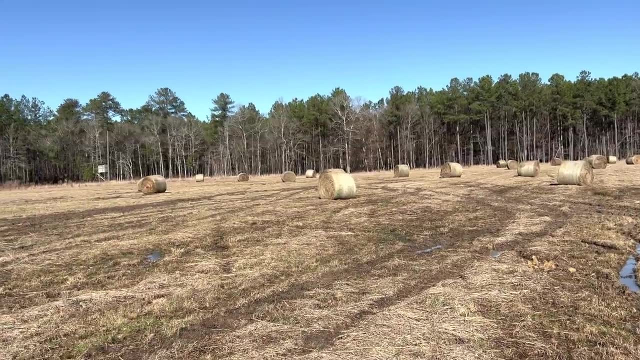 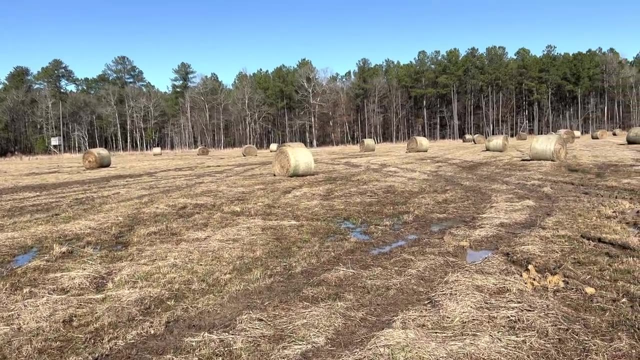 i'll set up some temporary poly wire and let the cows bail graze in this paddock. essentially, what bell grazing is is taking hay and either rolling it out or setting it out beforehand, whatever, and letting that cattle graze the hay. this field is so wet i. 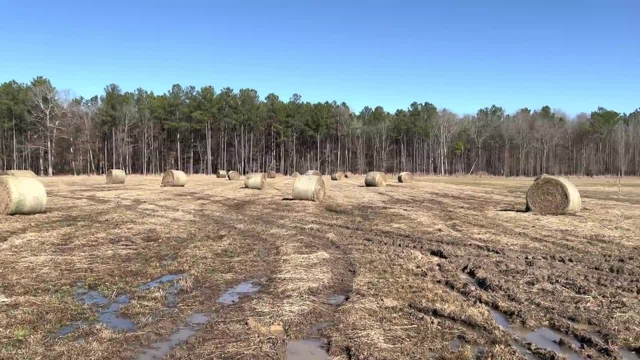 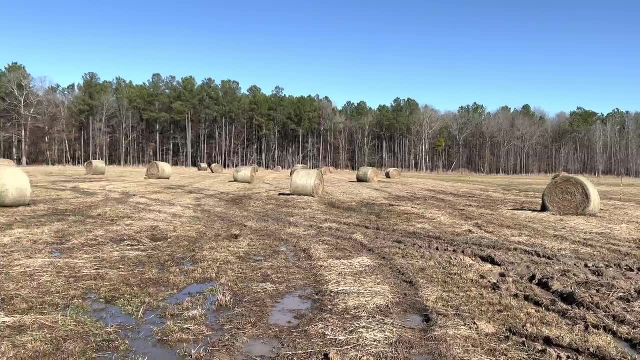 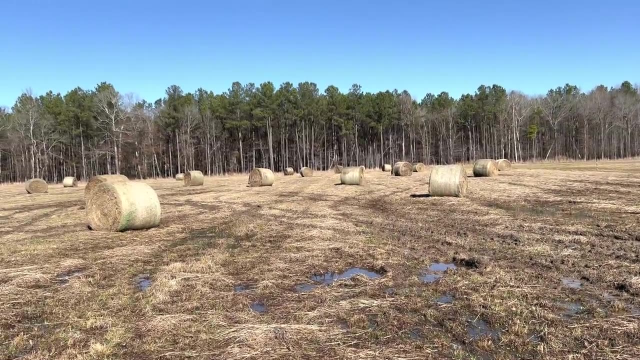 don't plan on unrolling the bales of hay, but rather we'll just take the net wrapping off, let the cattle graze. they'll manure a lot in this area and they will also leave behind remnants of hay. i've had a couple people reach out and ask me why we don't bail. 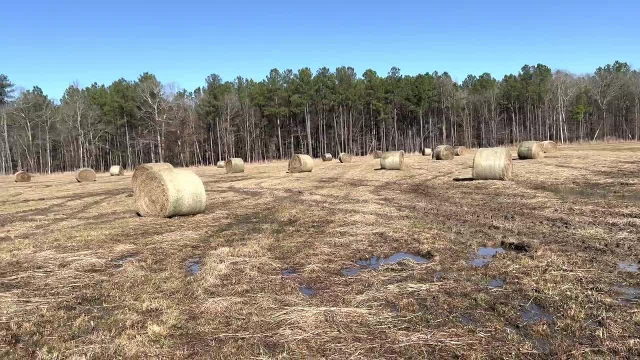 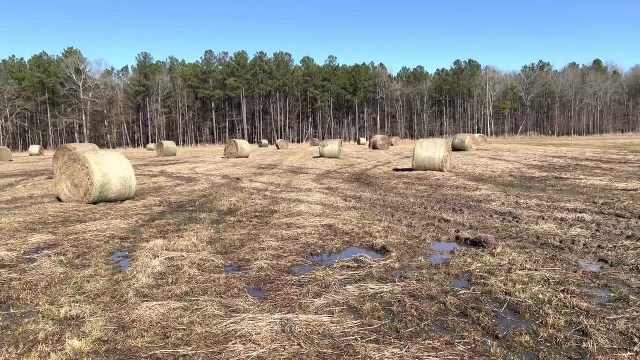 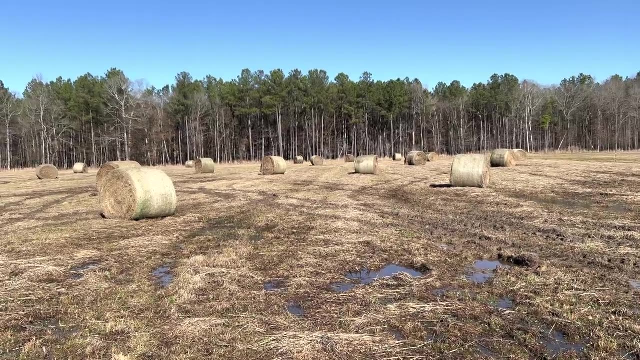 hay during the summer, when we have an excess, and the reason for that is quite simple. we only use 50 to 100 bales of hay per year and the cost of the equipment is just outrageous. when you get hay delivered for 30 to 40 dollars a bale- and it's decent, good quality hay. 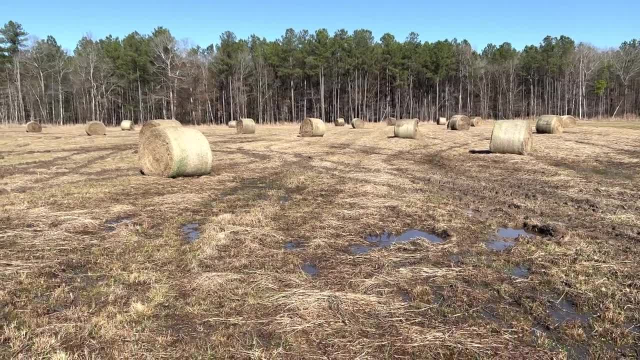 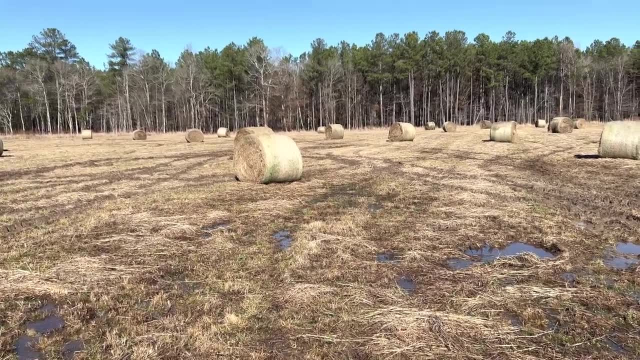 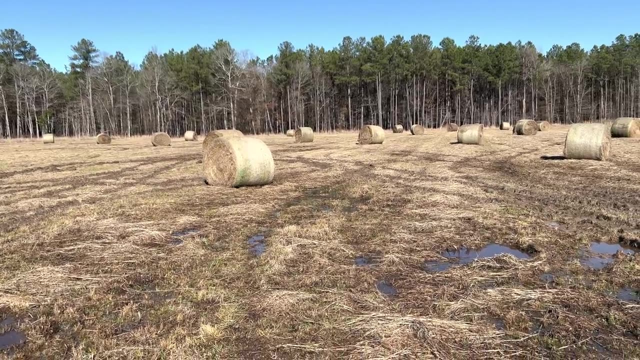 it's, we can purchase it cheaper than we could bail it on our own farm also out of. let's say we graze 50 bales of hay. that's a lot of hay in the field. that's easily 25 000 pounds of dry material that's being deposited. 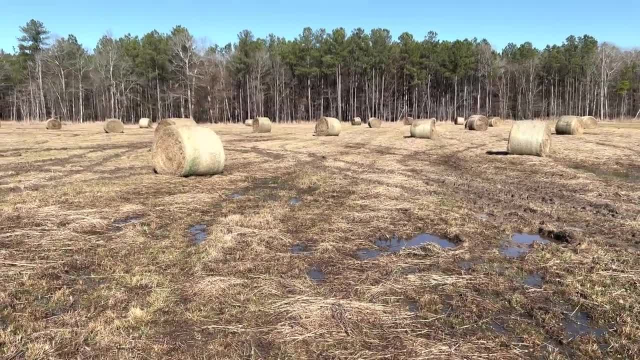 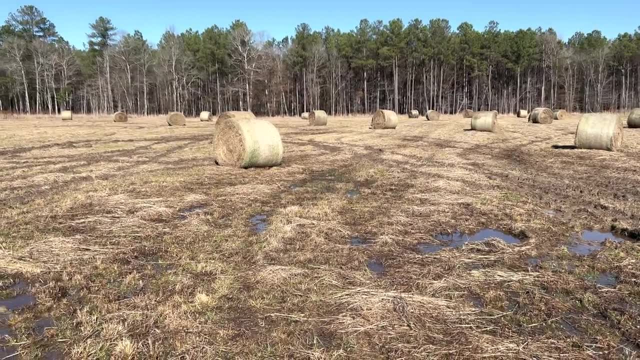 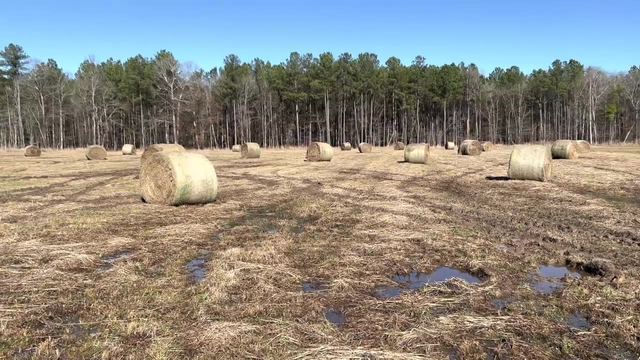 into the soil here on the farm. so we're importing those nutrients. it's good grazing for the winter. in an ideal world we wouldn't have to feed hay. but if we're going to feed hay, we'd rather buy it. it's cheaper than we could bail it ourselves, especially on a smaller scale. so later this week 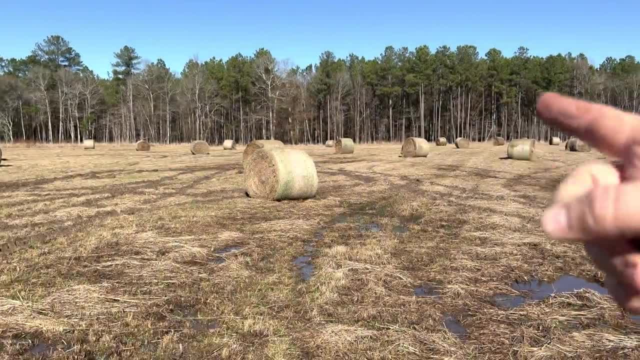 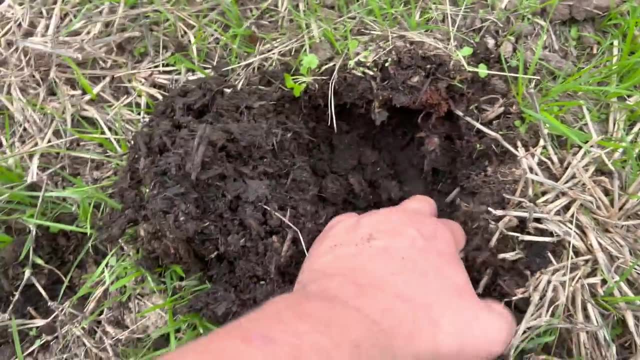 i'll set up, uh, some temporary paddocks and then we'll move the cows over here. so this is kind of what the soil looks like a year or so after pay is fed now the cattle, one of the things you'll notice is that, in bringing the hay, 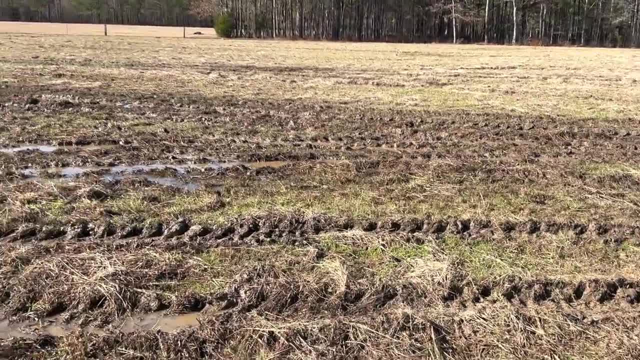 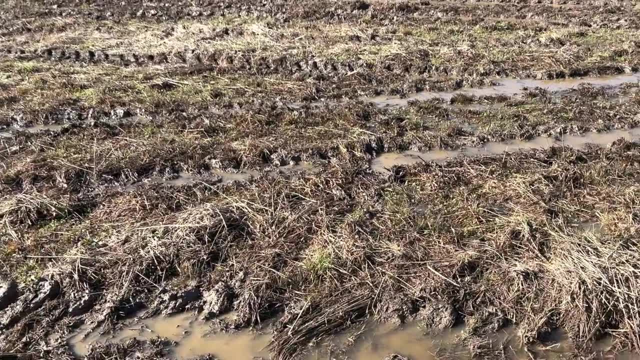 out here, especially while it was wet. i've had a world of a lot of issues with making ruts and all in the field, but again, keep in mind, the cows will be in here. they're going to trample this paddock to death. they'll destroy the sod. 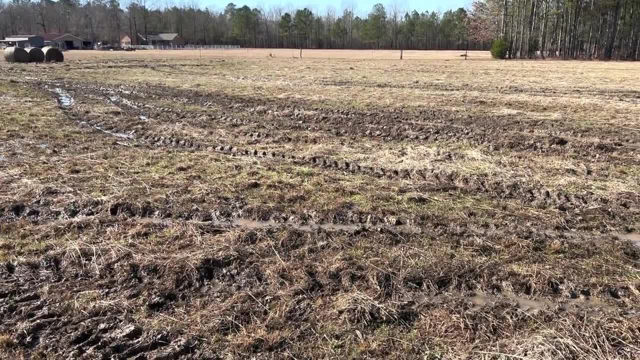 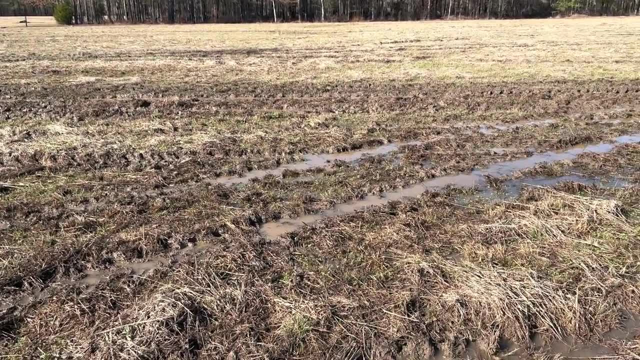 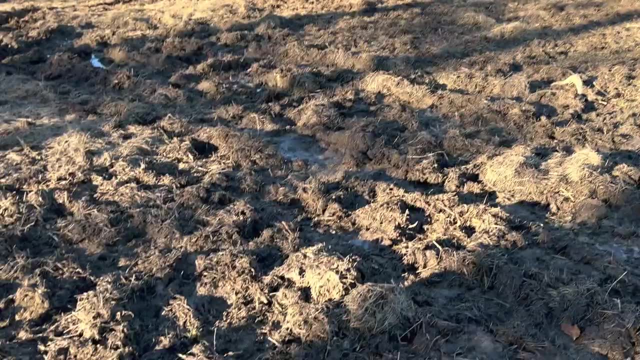 depending on the time of the year and the weather, i'll broadcast some seed winter peas or something like that. let the cattle kind of tromp it into the ground. the whole paddock will look worse than what these ruts are. it'll have manure and hay and straw and everything else mixed together and in that 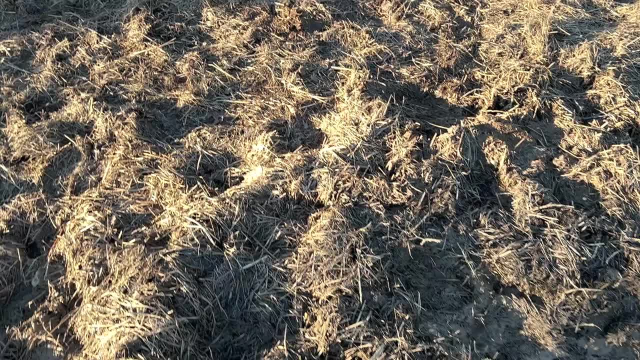 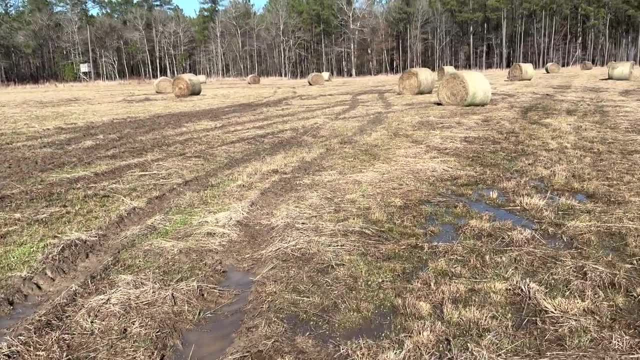 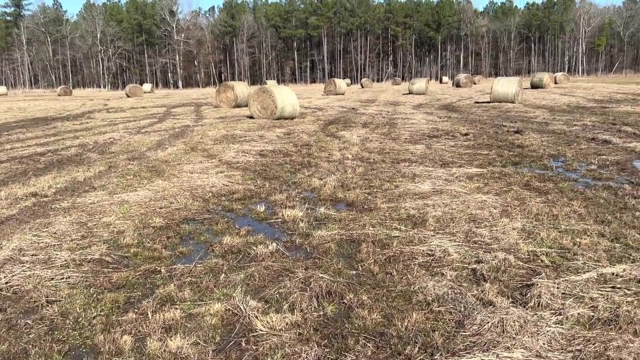 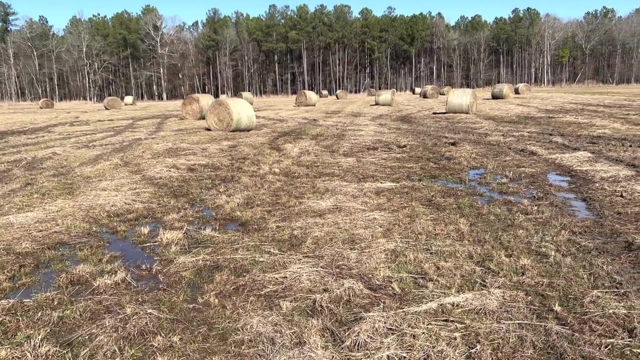 process. we can broadcast some smaller seeds and even some larger seeds into the paddock and it'll grow and, uh, put pigs in here again. the paddock is not level, it's rough to ride across anyway. and so with the pigs in here, with the forage cover crops, they'll get a lot of forage, they'll deposit a lot. 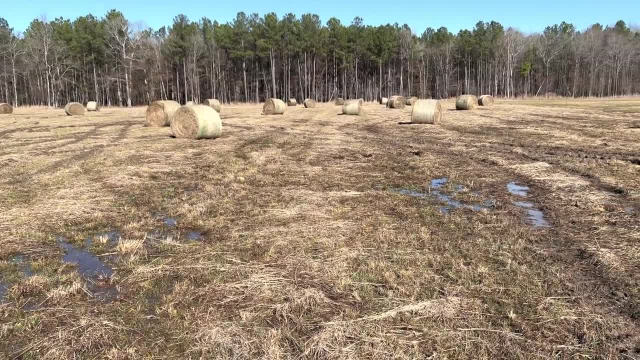 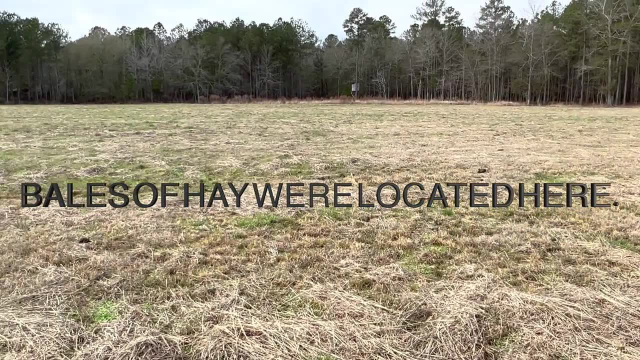 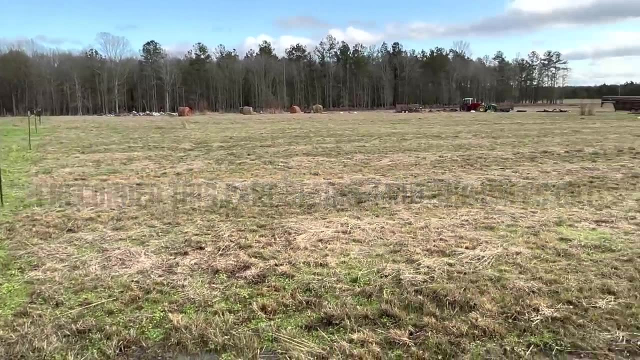 of manure and it'll increase the productivity of these 10 acres here as well. we're in the 10 acre field. this side to my left here is paddock a and this side to my right is paddock b. there's the tree line over there and then you probably can't see the fences. but over there 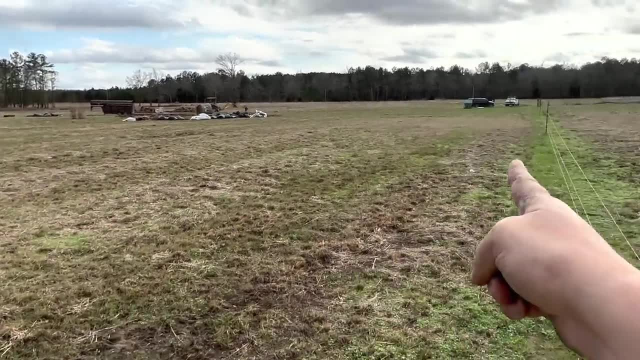 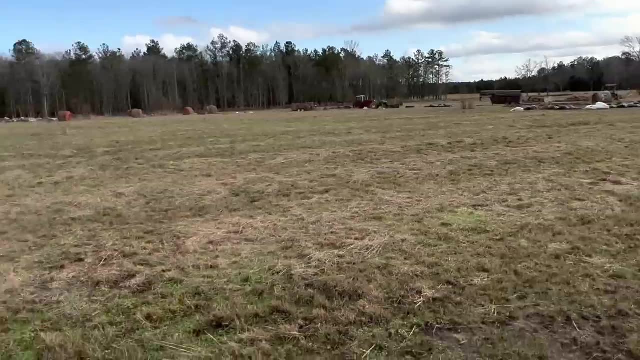 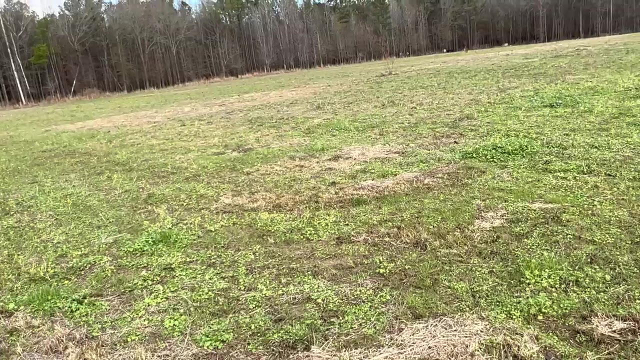 where the livestock trailer is, just this side of the tractor, just this side of that. those vehicles over there are where that this field stops. now the northern section over here to my left has been tilled and i grew some soybeans in it last august. they grew really, really well. i just did not get the 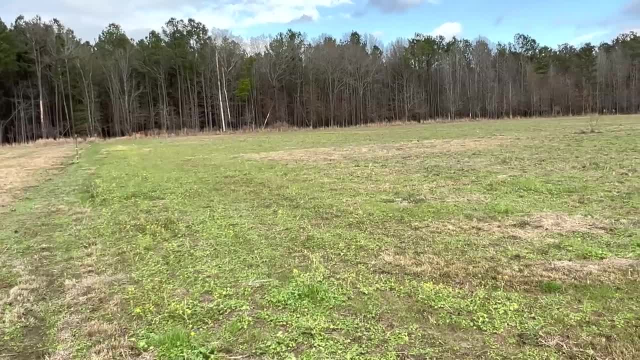 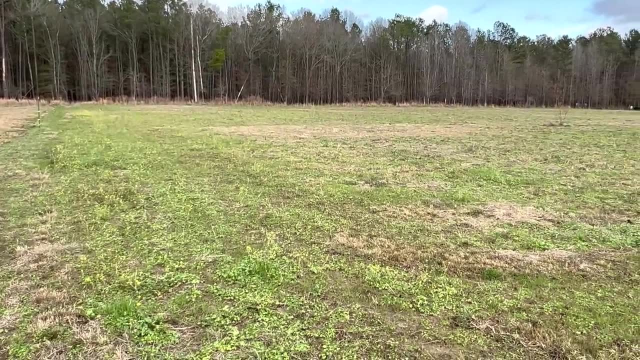 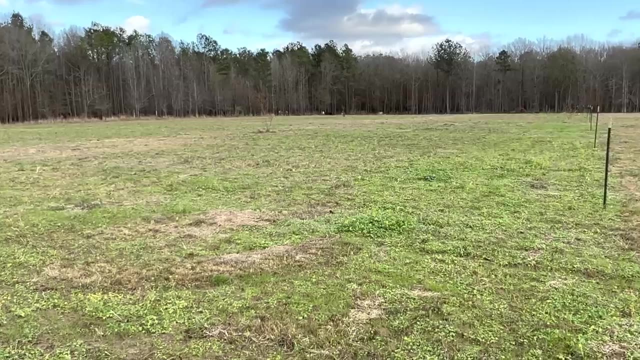 seeds out of the field. i didn't take them home. i had to raise them before the army worms came through and annihilated them. interestingly enough, i saw a flock of anywhere between 10 and 25 turkeys eating the army worms off the soybeans. the soybeans hadn't even gone to seed yet they 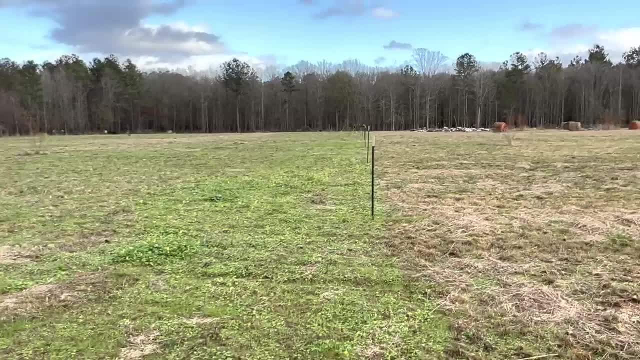 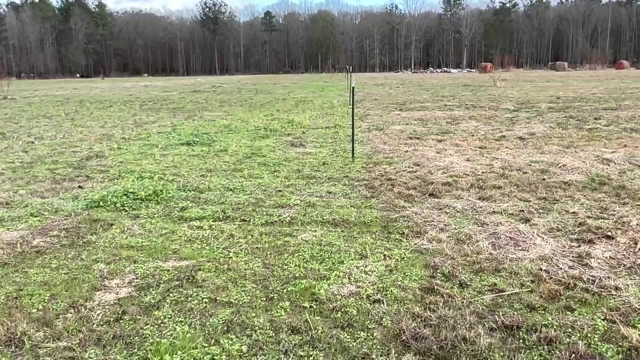 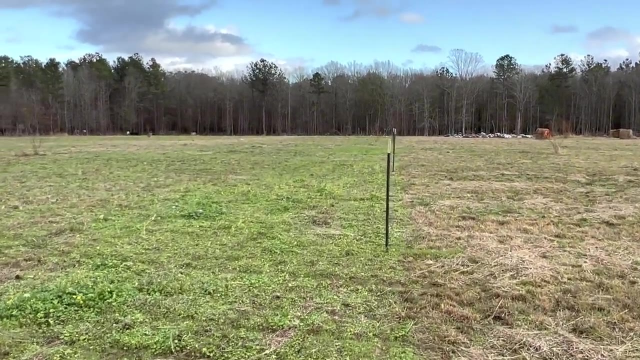 weren't eating the soybean seed, they were just eating the bugs off of them. so along the edge of where i've actually dished or tilled this field, here I have, And in the middle I kind of set up, a bunch of T-posts to put polywire. 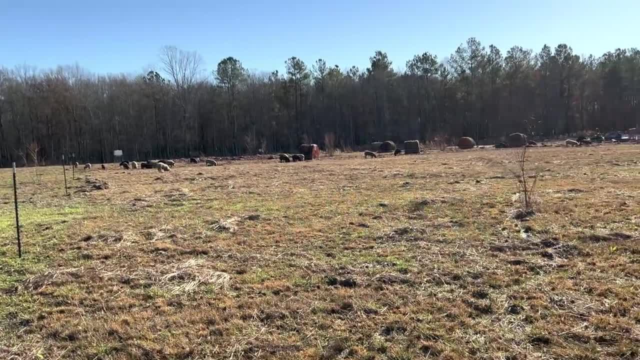 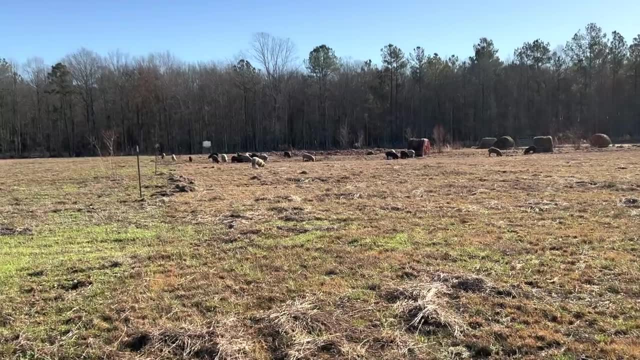 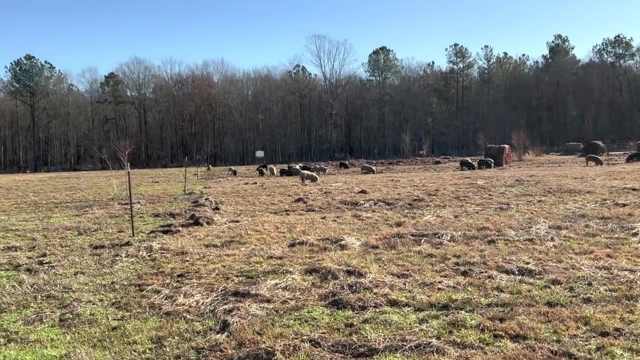 I just moved these pigs into this paddock. So as we begin looking east, as we are right now, the strategy in this field should become a little more apparent. My goodness, in the middle of filming we've got a mangalites, a pig. That's a bear that keeps jumping through. 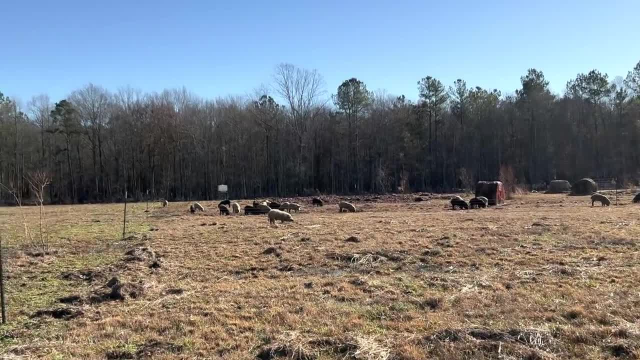 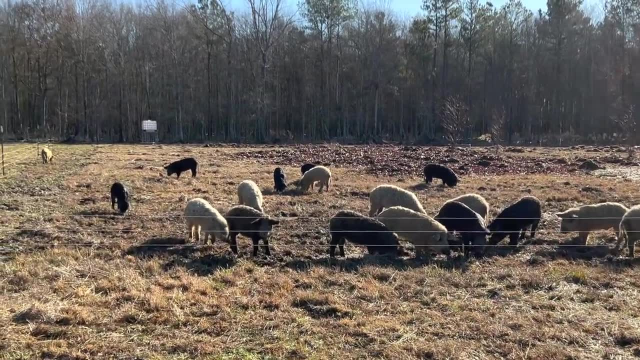 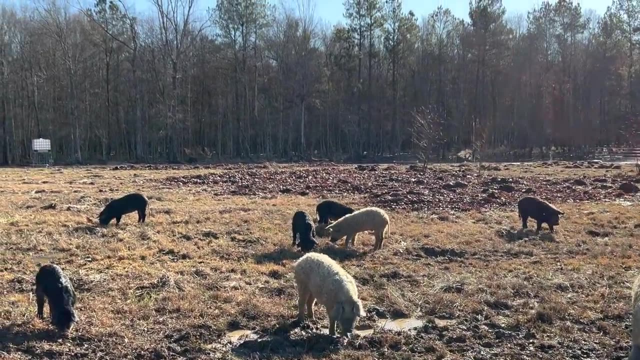 these electric fences. Anyway, things never go quite right on the farm. A friend helped me move these pigs into this paddock New Year's Day, and so the strategy is probably pretty obvious by now. We're applying mulches to the field directly. You can see that they're leaves. Again that same. 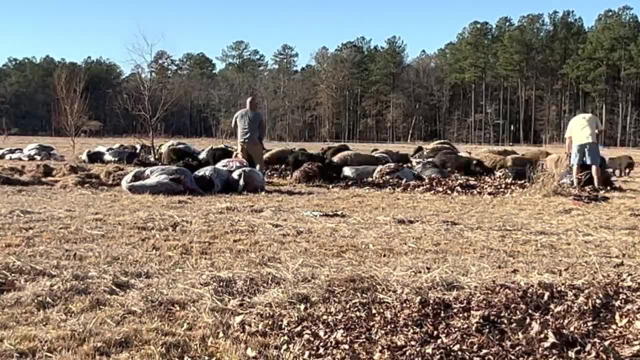 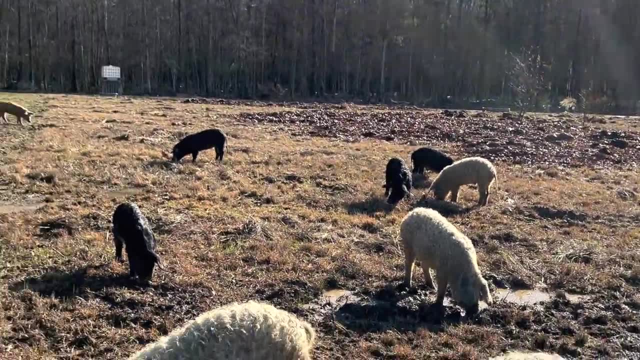 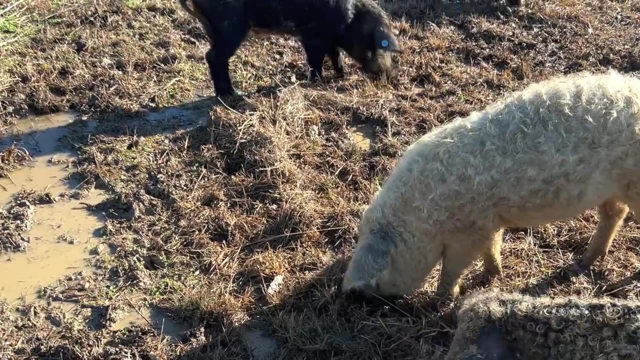 friend Bubba helped me put out about 100 bags of leaves or so Sunday afternoon. And then there's a bunch of mulch hay as well. We're using the pigs here to root up the sod. It'll save a good bit of tractor work. Yes, they'll make a few holes like this. 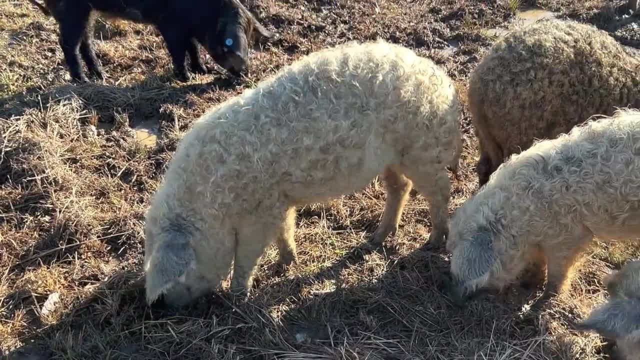 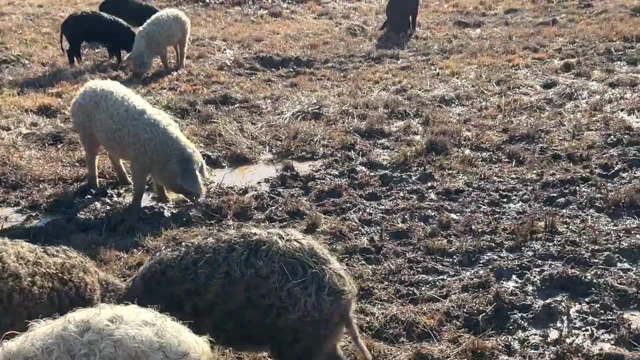 and the ground will be uneven. This time of the year they don't wallow too much. After all, it is January 4th and it's 60 degrees outside 65 degrees, so they're not going to wallow around. 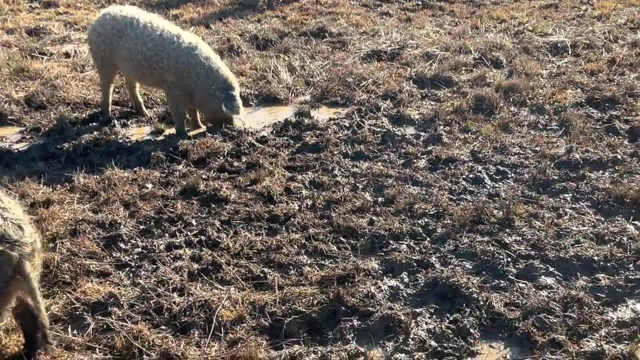 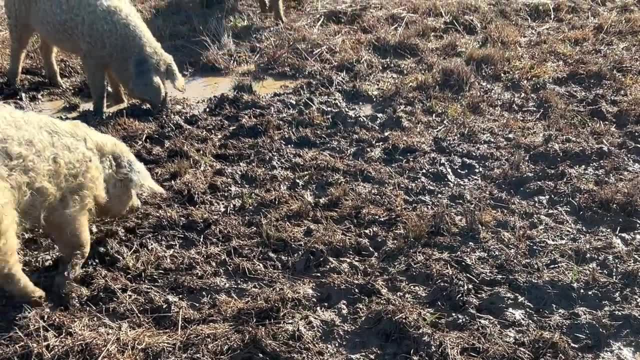 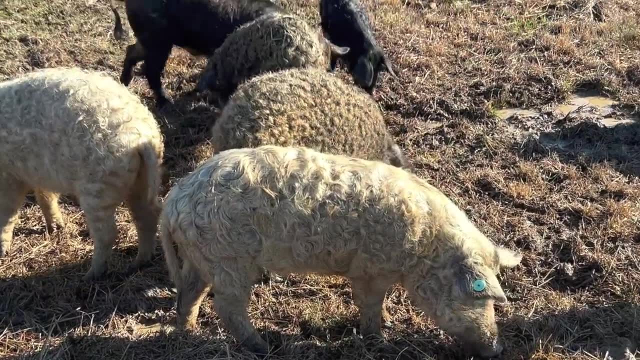 too much. You can tell where they've already rooted up a lot of the woody grasses, the cypress weed or dog fennel. They've also rooted up a lot of the broom sedge and the vases grass and so they're. 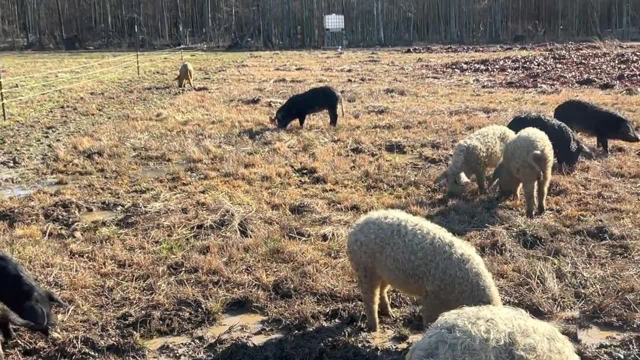 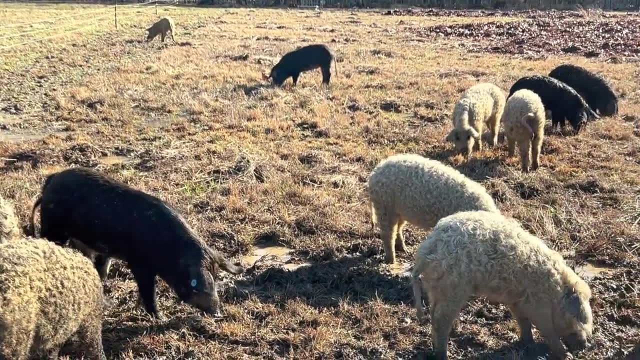 getting some forage and feed value out of it as well. But the biggest thing is that while they're out here they'll manure out probably 3,, 4,, 5, 6,000 pounds of manure in this field. That manure. 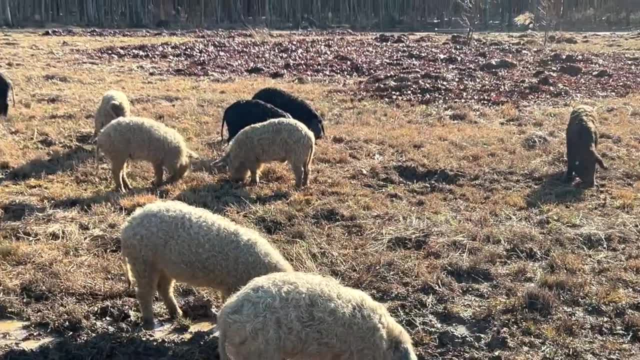 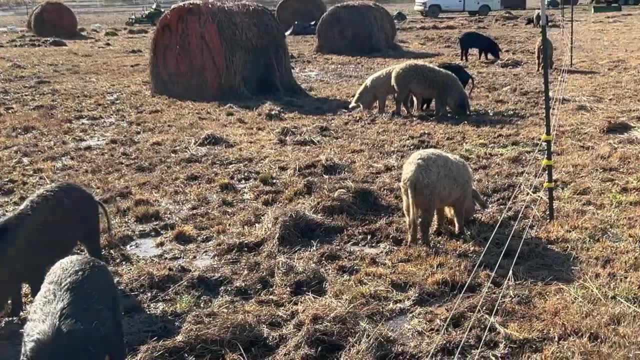 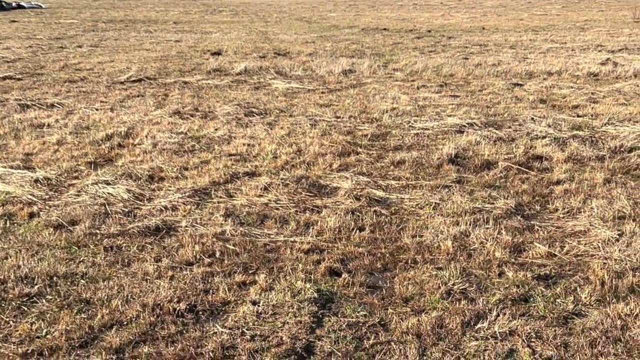 will build a lot of fertility in the soil. So in addition to the leaves and the hay, with the urea and the manure, there's just a world of a lot of benefit that the soil life will get out of this field. Now I'll move them down in further paddocks as well, and so they'll have two maybe. 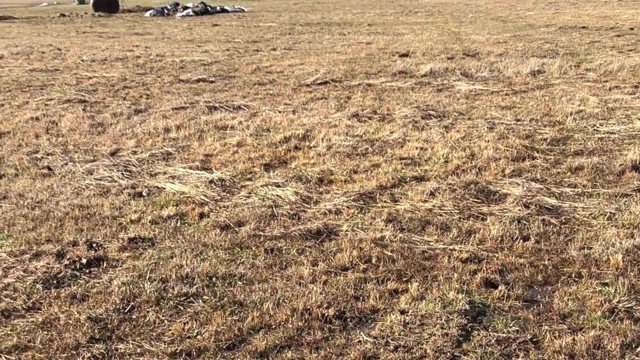 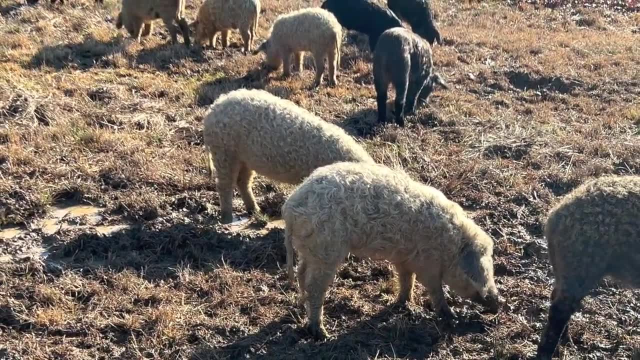 three more paddocks that I'll continue adding mulches to the fields. Then I'll fence them in and move the pigs there as well. So before I move the pigs I'll broadcast cover crops That'll serve three or four different purposes. First and foremost there'll be ryegrass and or. 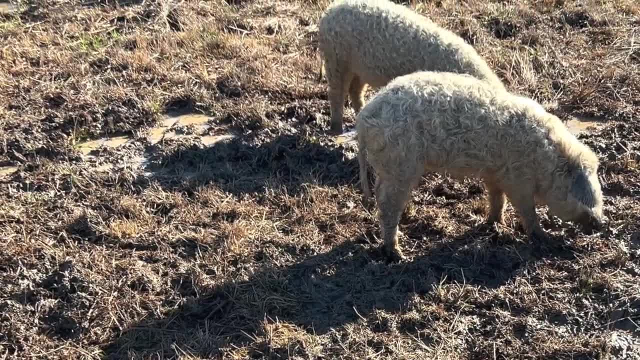 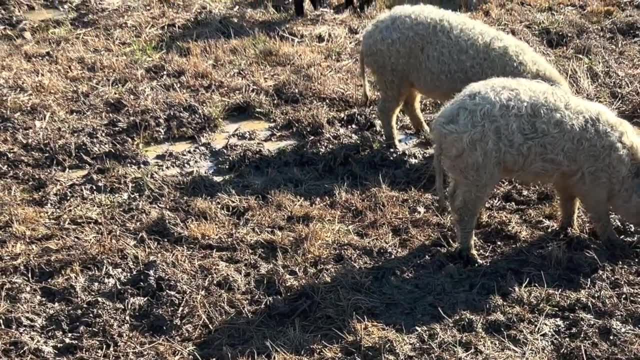 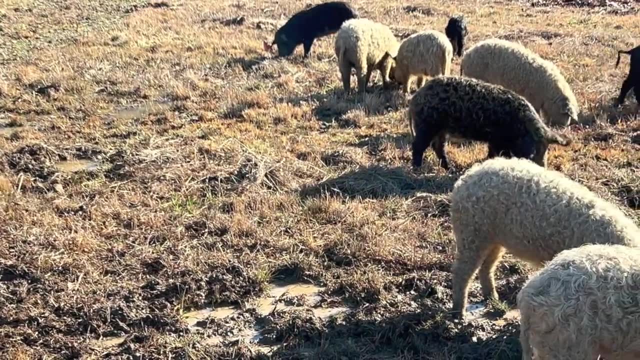 cereal rye. that'll help absorb the nutrients in the soil right now. They'll both grow really well in our winters here, but I'll also include some legumes like clover or Austrian winter peas. The legumes will help fix additional nitrogen and also provide a higher protein feed for the. 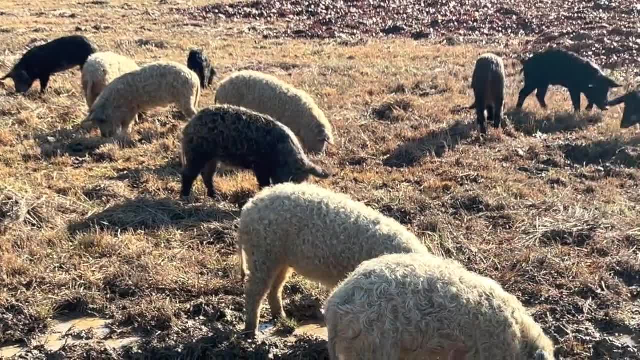 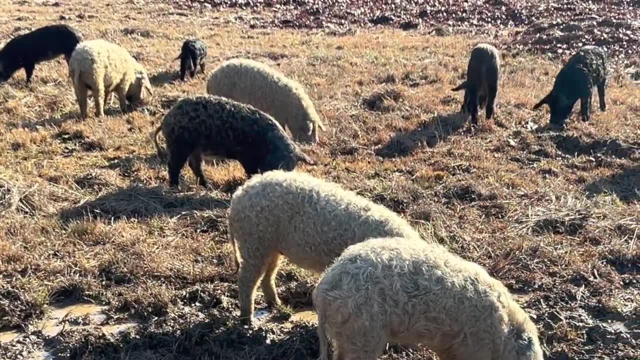 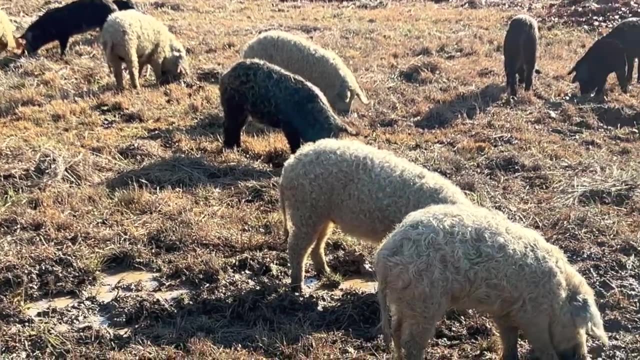 pigs when I move them back in here again in March or April or May. But I'll broadcast the cover crop seeds two or three days before I move the pigs. I'll make sure that they're not treated and I'll broadcast them at two or three times the normal rate and then I'll bring them, leave them there for a couple of days. 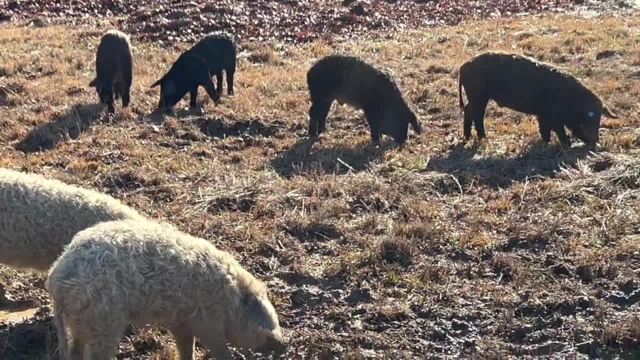 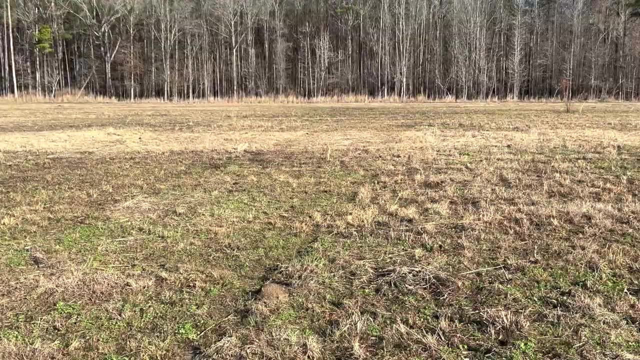 The pigs will eat some of them, They'll trample a lot of them, They'll miss a lot of them, and then I'll bring the pigs over to the next field. In the northern side of the field I've already planted clover and ryegrass. and ryegrass should do relatively well. You can see little bits of strains of ryegrass. We just had a real, real, real cold weather for our area: Eight degrees no snow on the ground. So the cool season crops were killed, Their growing points. 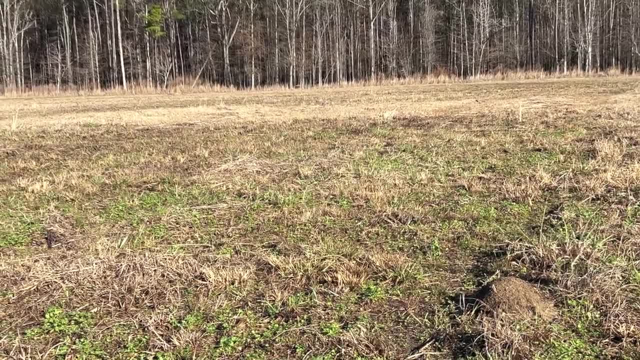 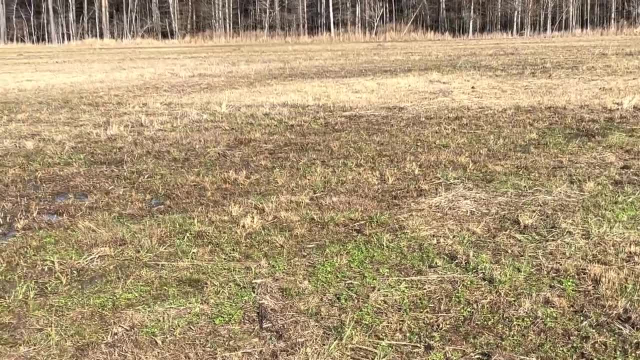 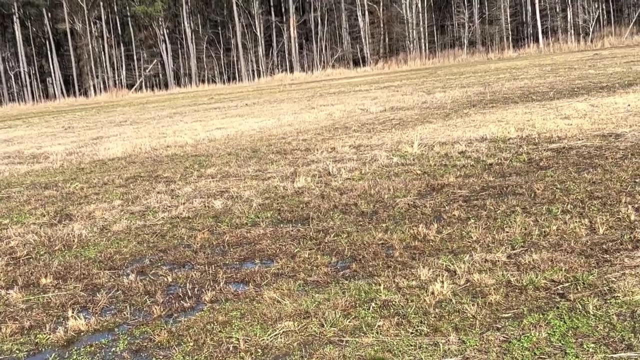 were not, so they'll grow back. But the clover will grow pretty well And this field will have a lot of forage value in it this spring, hopefully. Even if it doesn't, I can still put the pigs out here. They'll get some feed. 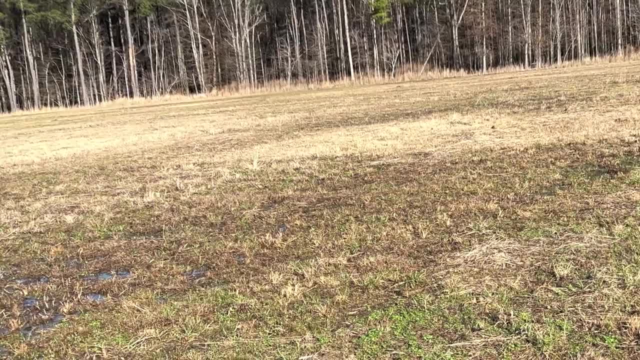 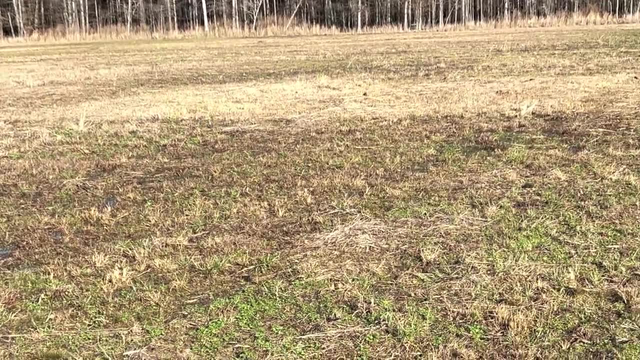 value out of it, just not as much. And then I'll broadcast warm season cover crop mixes that include sorghum, sudangrass, millet, cowpeas and that kind of stuff. This strategy in the field will help reduce the amount of equipment.